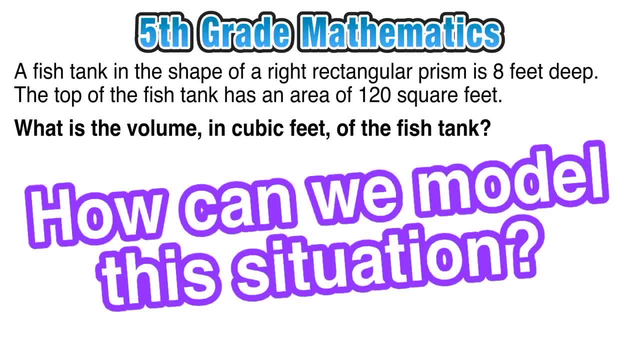 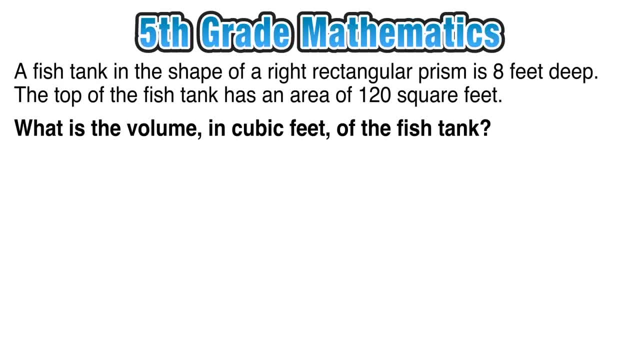 diagram and take our thoughts and put them onto paper, we can much better understand what's going on here and better find a solution. So remember that our fish tank was in the shape of a right rectangular prism and we know that the volume in cubic feet of the fish tank is eight feet deep. 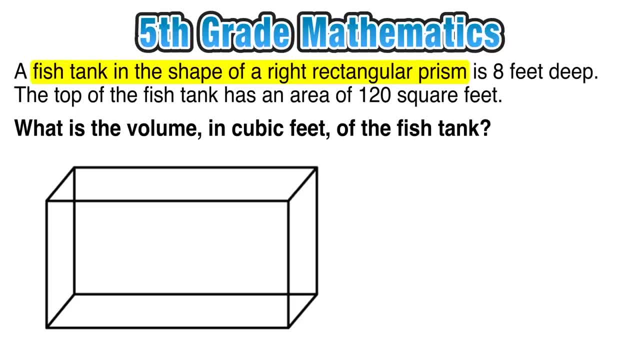 We know what that looks like, except it is a fish tank. so let's fill it up with water and add a few fish, And we know that the fish tank is eight feet deep, so we can go ahead and label that depth on our diagram. Now, remember that we wanted to find the volume of this fish tank and we 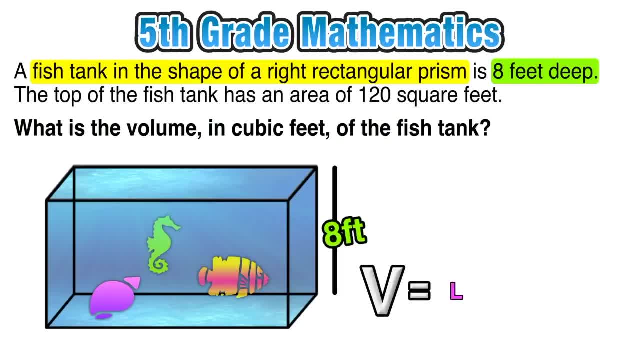 know that the volume of a right rectangular prism is length times width times height. Now, so far, we only know what h is, We only know that the height of the rectangular prism is eight. We don't know the length and we don't know the width, But what we do know is that the top of 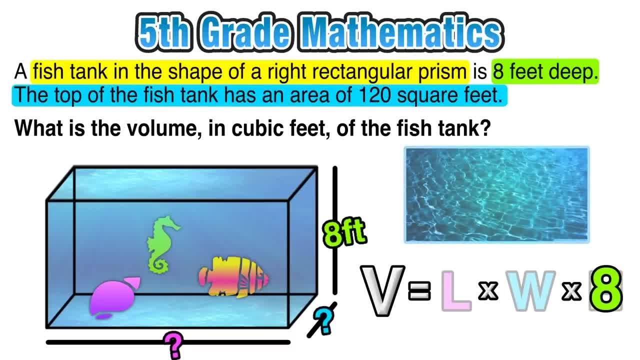 the fish tank has an area of 120 square feet. Now, the top of this fish tank is just a flat rectangle and we should already know that the area of a rectangle is just length times width. So whatever the length times width is is going to equal the area, and we already know that l times. 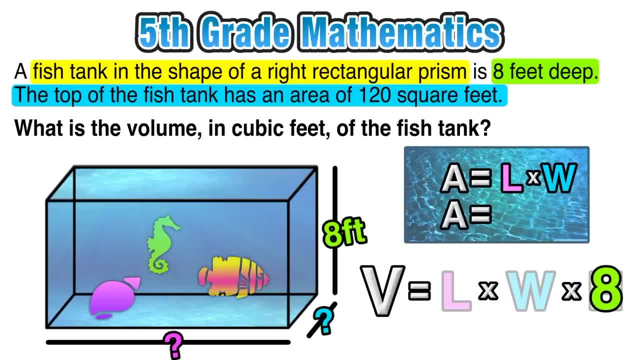 w for this particular shape is going to equal 120.. So even though we don't know the exact measurements of the length and width of the fish tank, we know that their product is going to be 120.. So remember that in the volume formula we didn't know what l times w equaled. Well, now we do. We know. 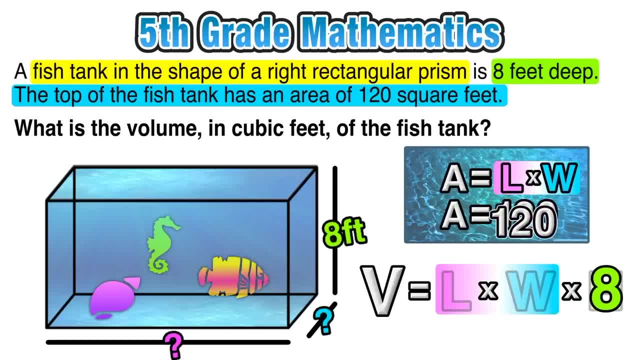 that length times width equals the area, and we already know that the product is going to be 120.. length times width for this rectangular prism is 120.. So I can slide that right into the volume formula. So now I can say that the volume is equal to 120 times 8.. And the product of 120 and 8